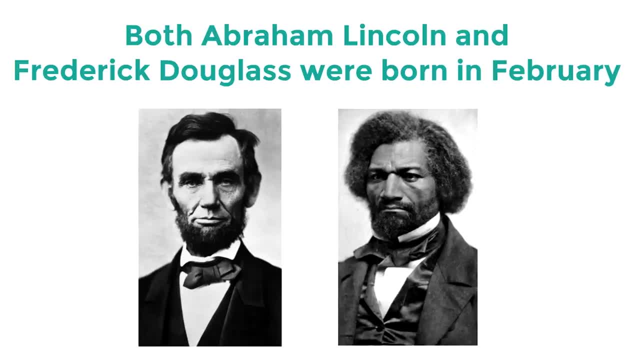 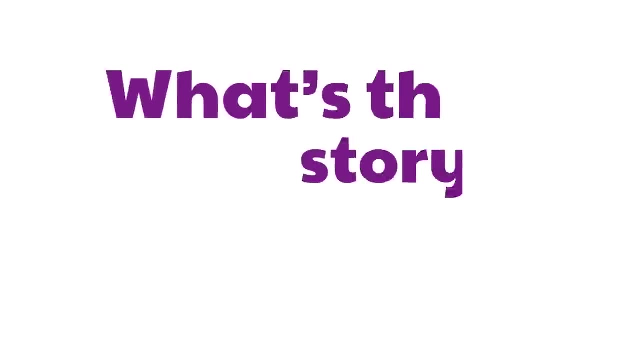 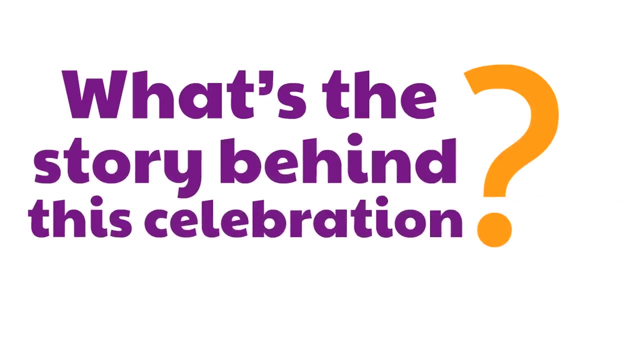 And so many other people worked to that end too, But Abraham Lincoln and Frederick Douglass were some of the main figures in ending slavery. February is the perfect month to celebrate Black History. Okay, so what's the story behind this celebration? Well, it all goes back to this man, a man named Carter Woodson, who would later be known as the Father of Black History. 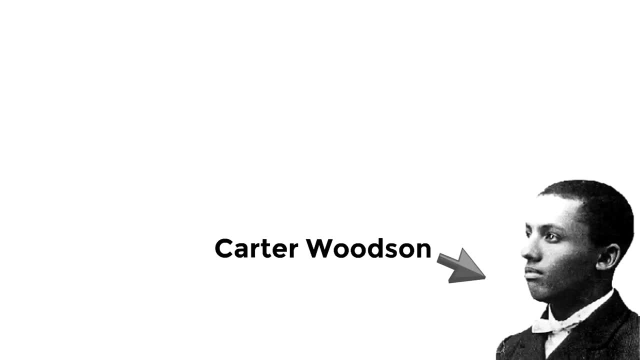 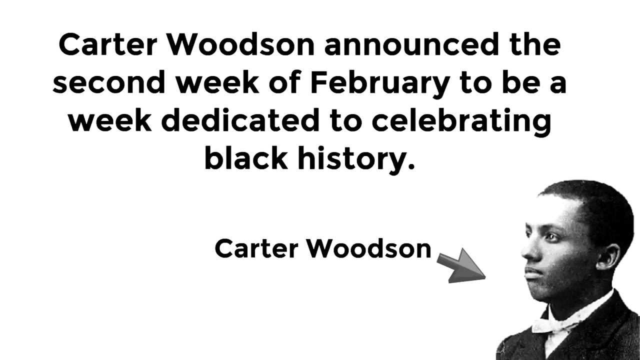 He was a historian and a well-published author who was concerned that the stories of Black History were not being told. Carter Woodson announced the second week of February to be a week dedicated to celebrating Black History. You might say a week, It's a month, It's Black History Month. 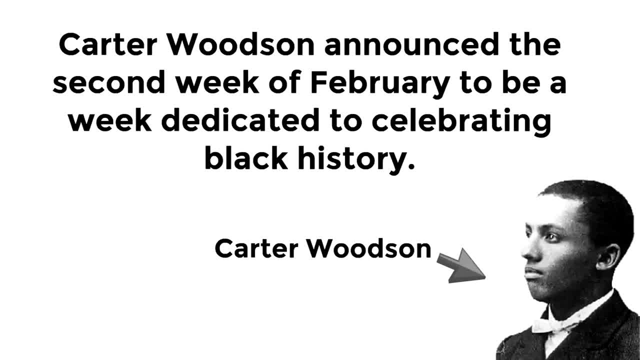 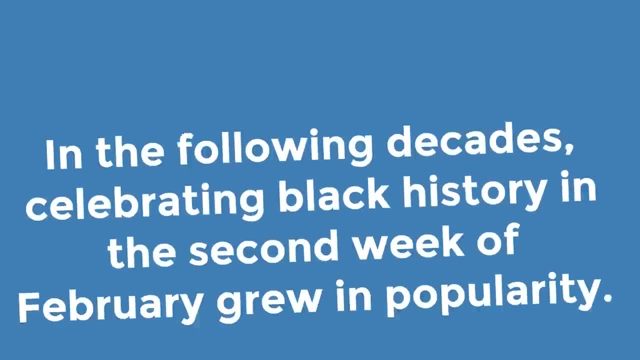 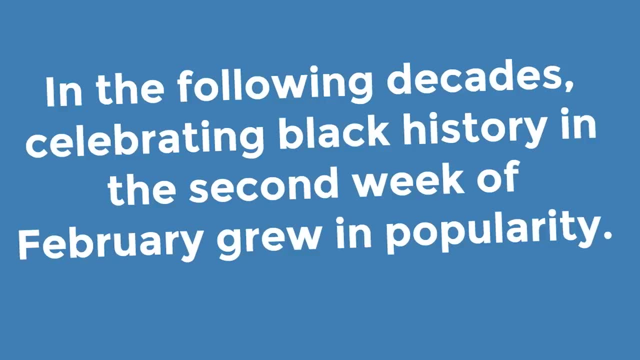 Well, you have to hold on. At first it was just a week. It was the second week of February. In the following decades, celebrating Black History in the second week of February grew in popularity. More and more people were celebrating Black History on the second week of February. 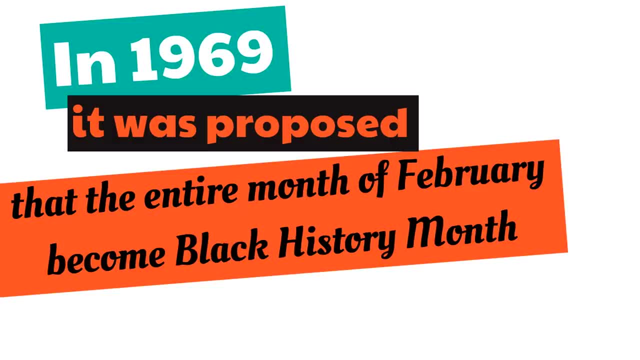 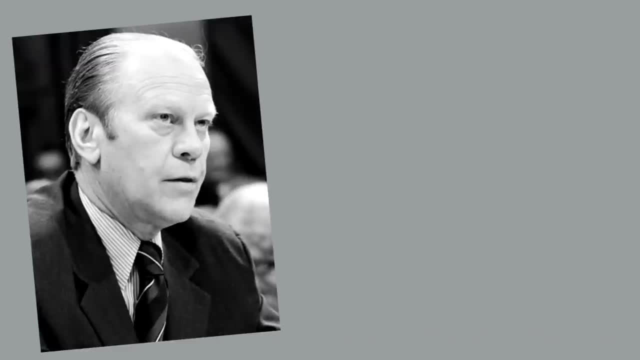 Then, in 1969, it was proposed that the entire month of February be celebrated as the second week of February And that the month of February become Black History Month. Then, just six years later, in 1975, President Gerald Ford recognized Black History Month. 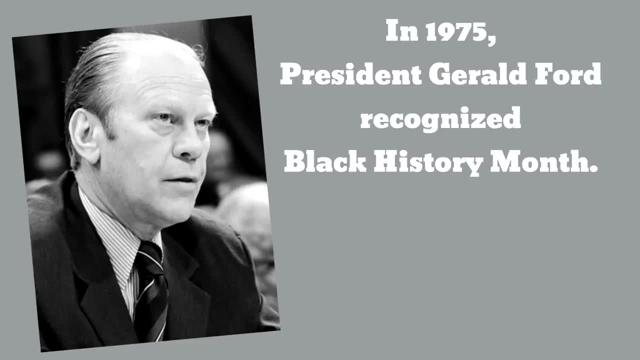 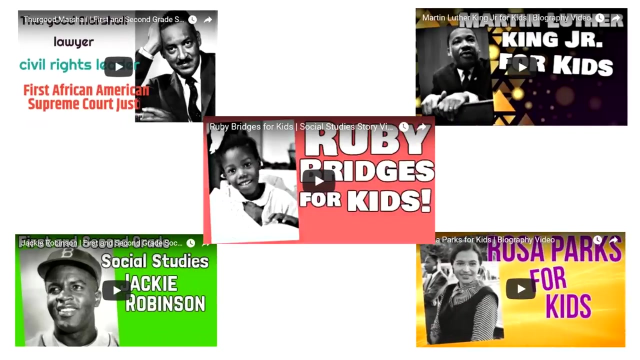 He said officially, listen everybody, this is a thing. the month of February, it's important to celebrate Black History. He said the accomplishments of African Americans have been too long neglected. That's why here on Homeschool Pop, we've featured some of these incredible stories of men and women of African American descent who have made a huge impact on our world. 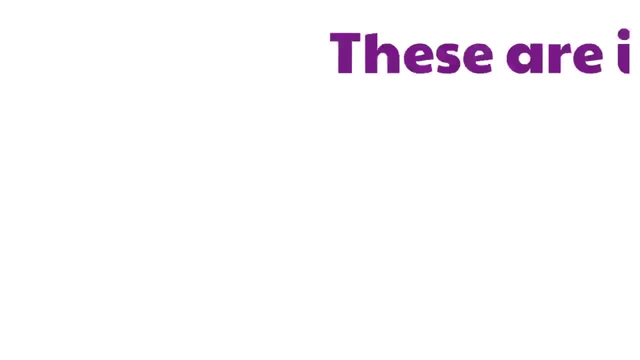 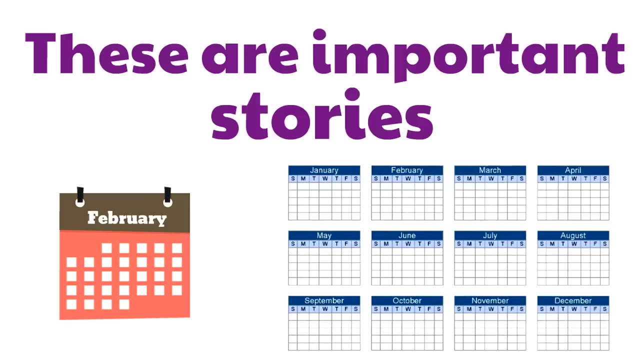 The thing you have to remember, though: these are important stories. They're not just for one month, not just the month of February, Black History Month- but it's for the whole year. These stories are to be cherished, and they're important.